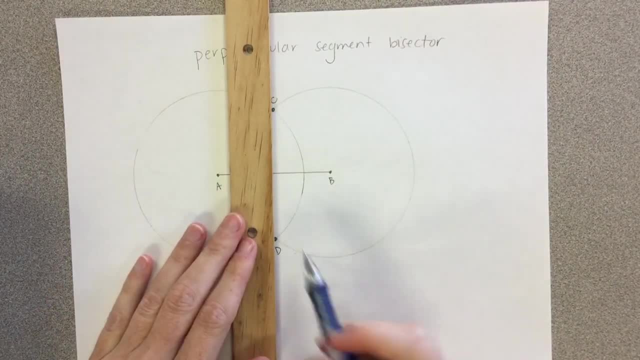 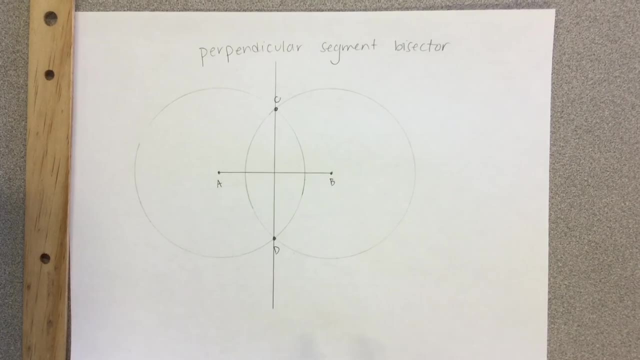 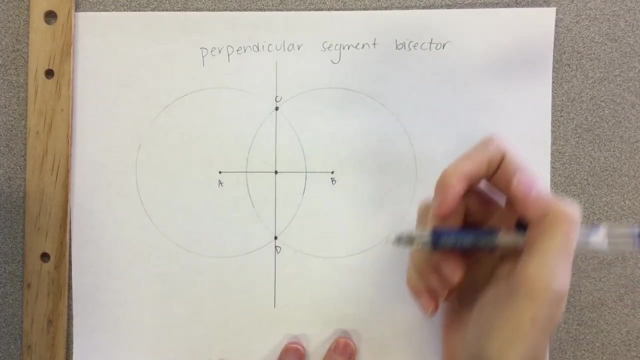 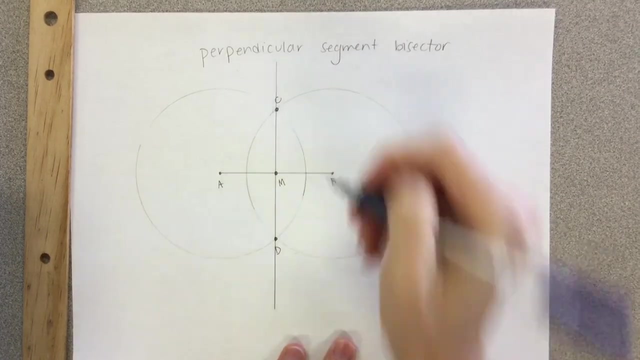 my straightedge. I'm going to draw a line connecting points C and D And this line that I just drew in where it intersects our original line, segment AB. that point is the exact middle of segment AB. I'm going to call it M for. 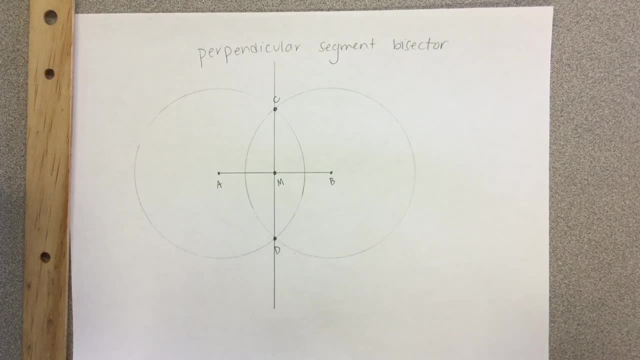 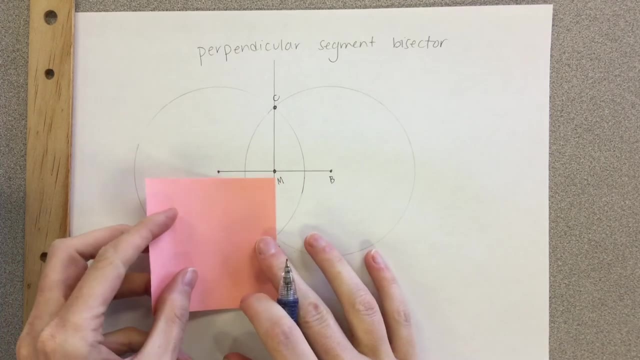 midpoint. So one way that I can check that, that I can confirm that it is the middle and still, without using any numbers, I'm going to use another little piece of paper, and what I'm going to do on this paper is I'm going to mark the 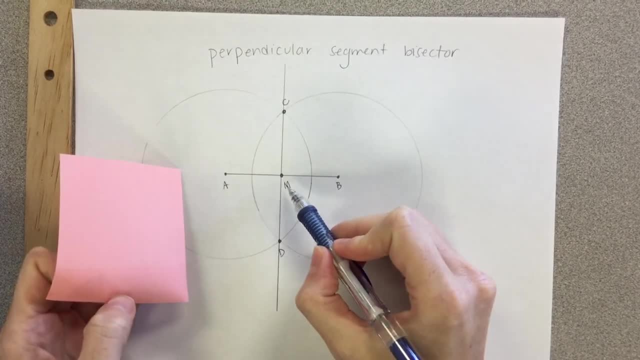 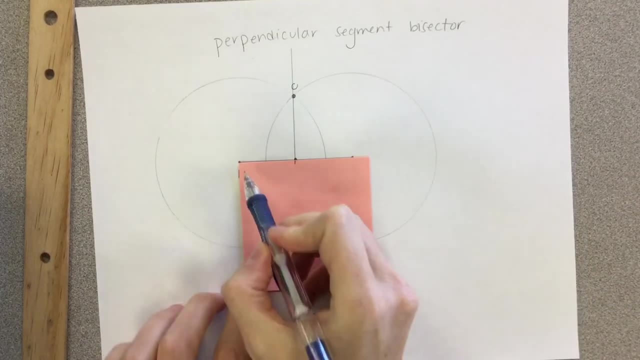 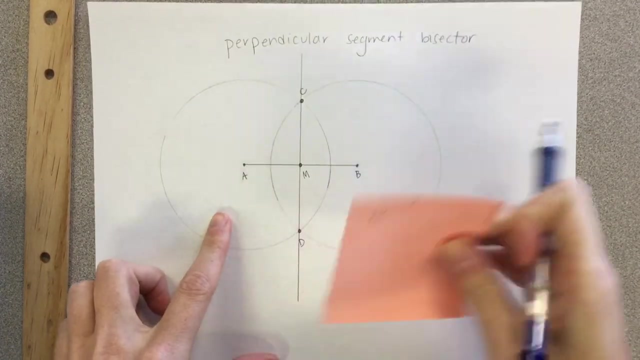 distance from point A to point M, the midpoint, And then I'm going to check to see that the same length as from B to M. So this distance right here is the length of line segment AM. So now, if I move my little piece of paper I can see. 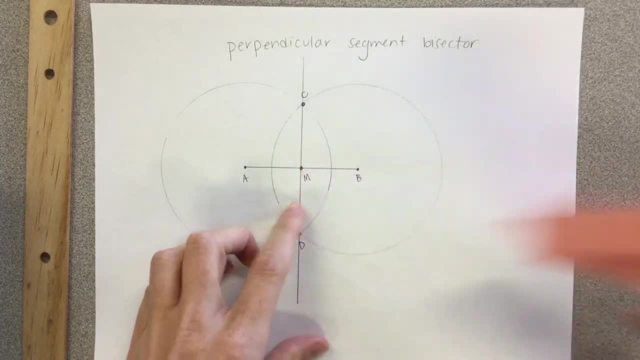 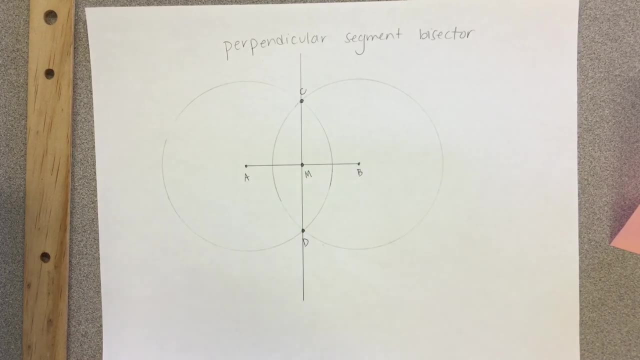 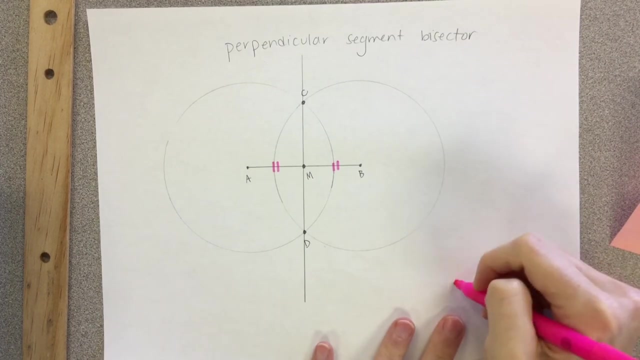 that that is the length of segment AB. I'm going to add another piece of paper the same length as segment BM, And so I know that AM and BM are the same length and I'm gonna put little congruent marks on those segments. I know that AM is. 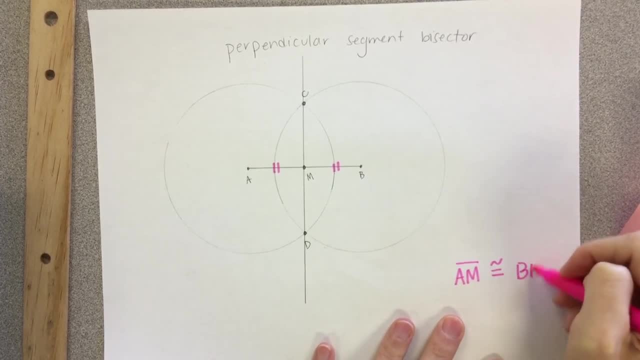 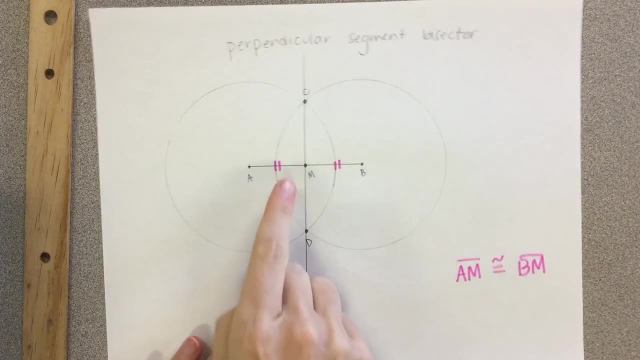 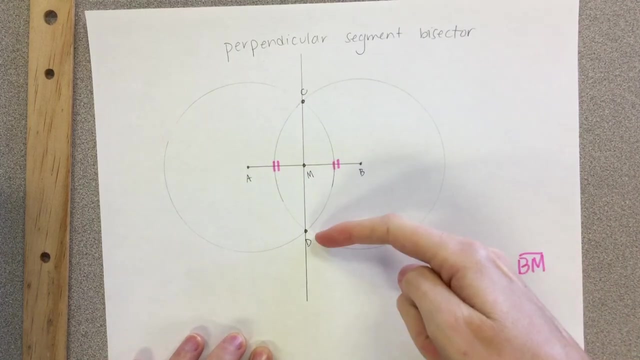 congruant to BM. Now you may also notice that these angles here, these four angles that are formed from the intersection of segment AB and segment CD, these kind of look like right angles. So I can check that Again. I'm going to use my little. 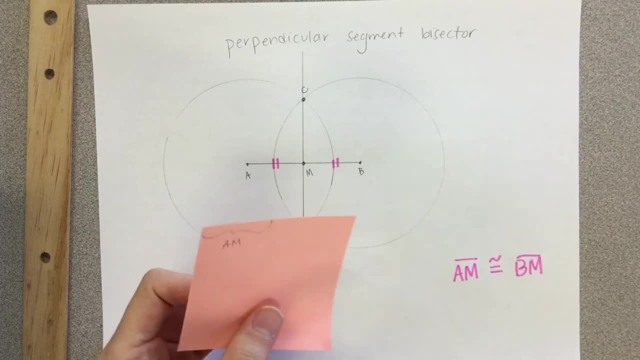 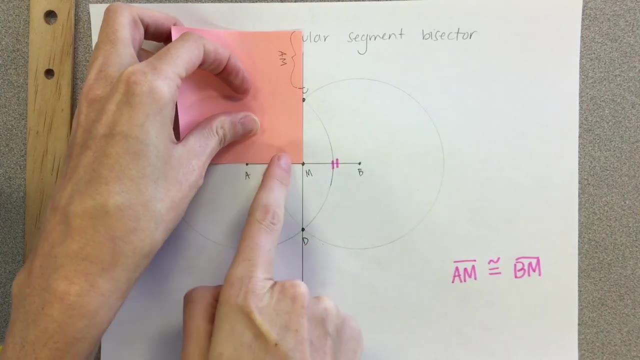 piece of paper. I know that on this piece of paper, each of these angles is 90 degrees. And so if the segment AB is congruent to BM theseن, And so if I put a corner of my little piece of paper in one of these angles, yeah, it is exactly 90 degrees. 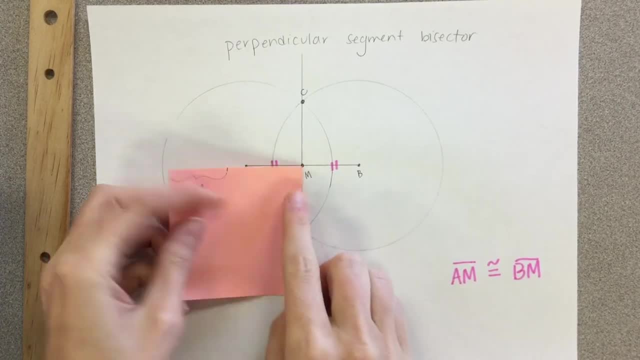 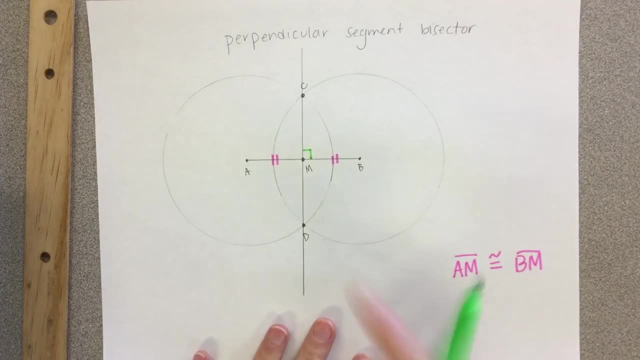 And I can check that for each of them, Each of these four angles here is 90 degrees, And so I'm going to put a little box here to show that that angle is 90 degrees, And so is this one and this one and this one. 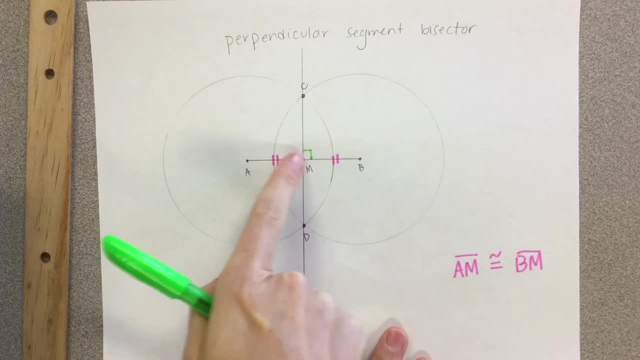 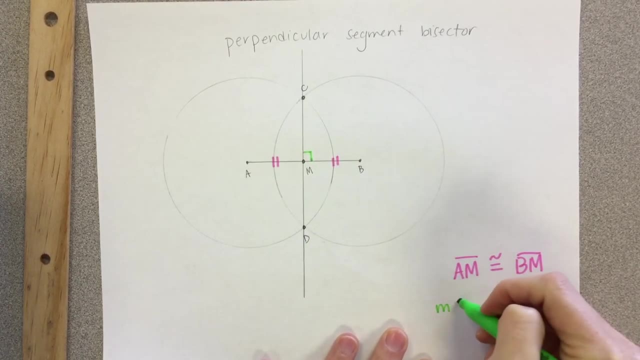 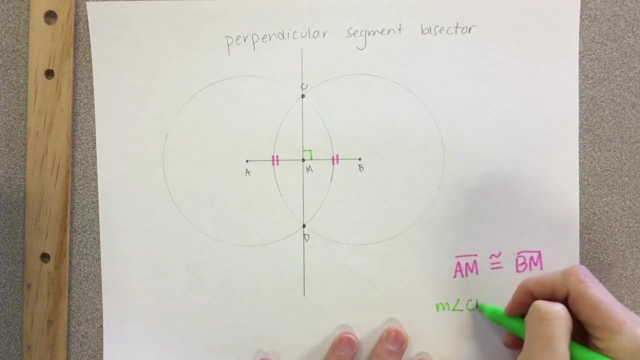 And so I could write a statement over here to say that one of these angles is equal to 90 degrees. The way that I would write that is I would write M for measure of angle, And this would be angle CMB is equal to 90 degrees. 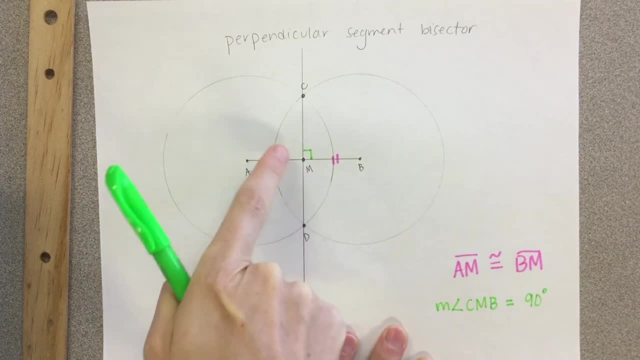 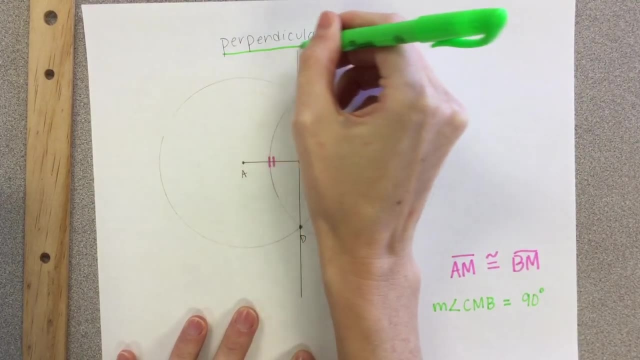 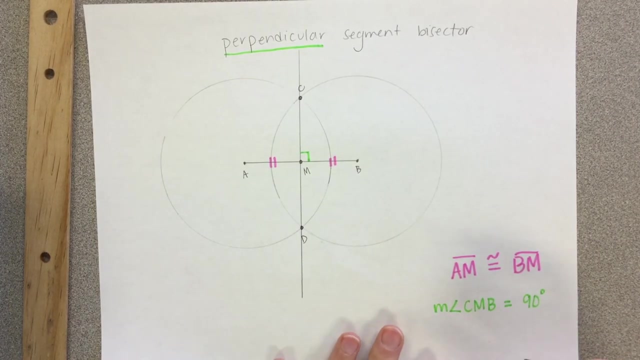 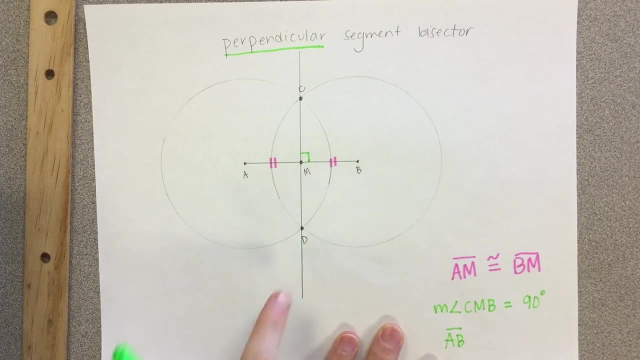 And I could write a statement like this for each of these four angles in the center. Now this word perpendicular. this means that two lines intersect at 90 degree angles. So I could also write that segment AB is perpendicular to segment CD. 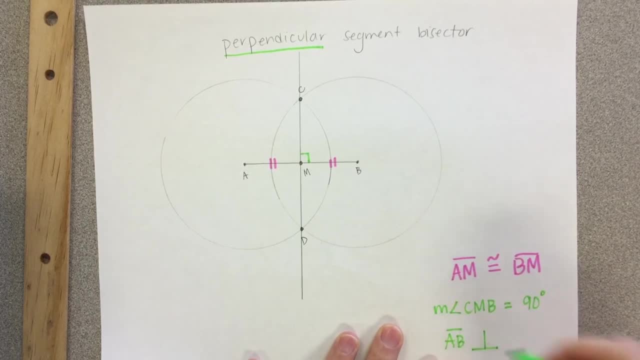 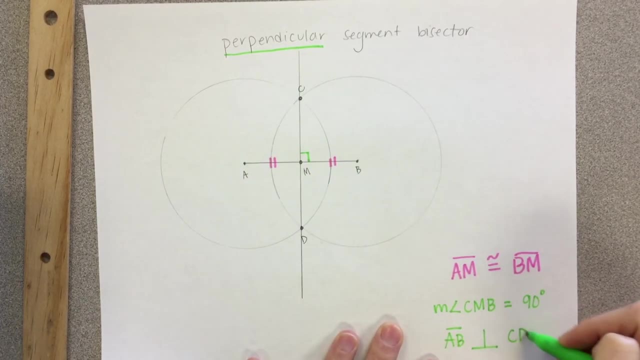 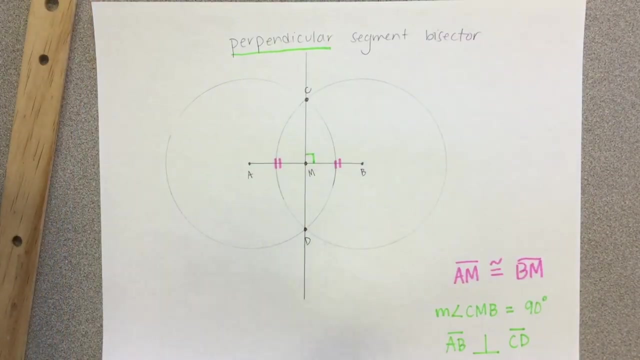 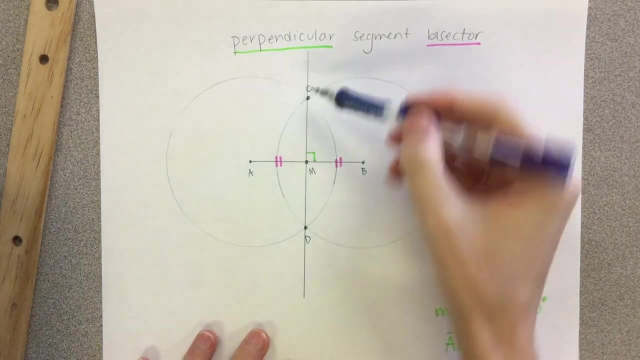 And the symbol for perpendicular is like an upside down T, So AB is perpendicular to CD. Now, going back to our original title up here: perpendicular segment bisector. bisector means to cut in half, And so this line here, CD. this is our perpendicular segment bisector. 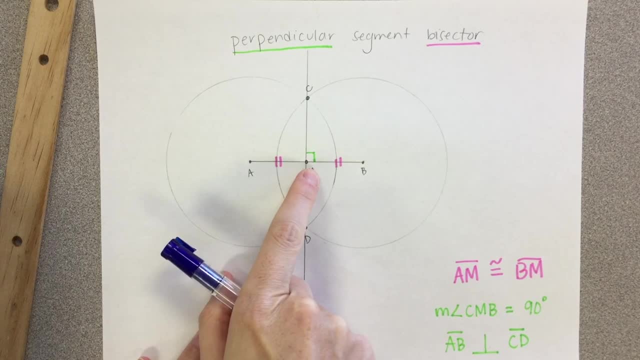 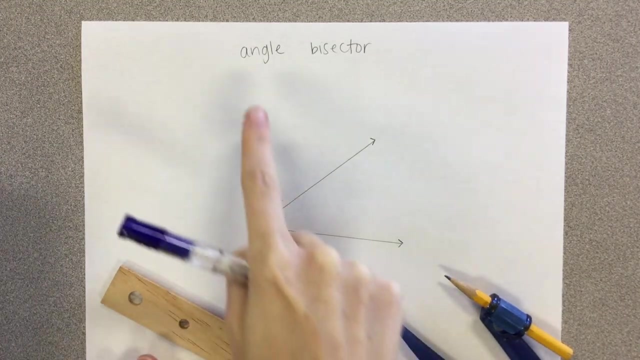 It's perpendicular because it forms 90 degree angles, And it's a bisector because it cuts segment AB in half. It creates two congruent segments. Next, we're going to construct what's called an angle bisector, And so I've already drawn an angle here using my straight edge. 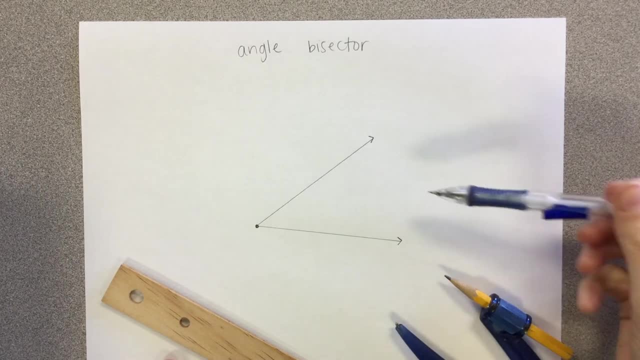 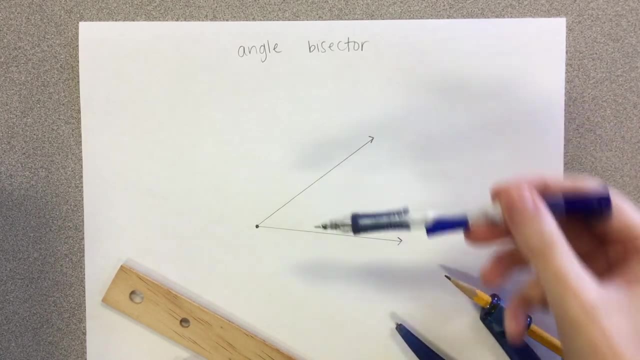 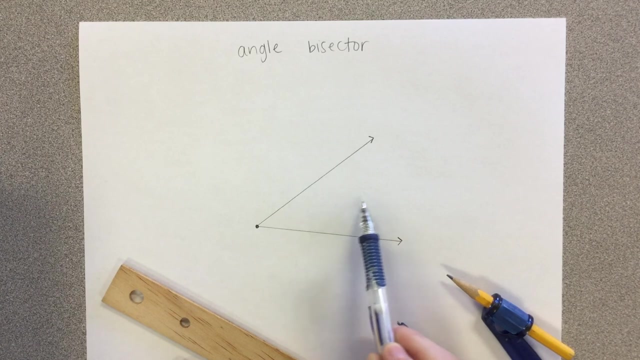 And so what we're trying to find is the exact middle of this angle, meaning we want to take this big angle and cut it in half, cut it into two smaller angles that are equal size, that are congruent. So again, I could kind of estimate. the middle seems to be about like right here: 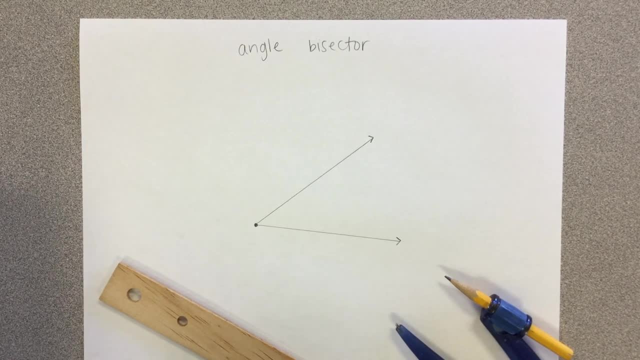 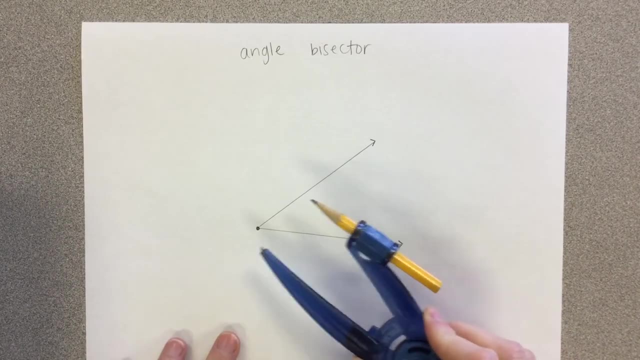 But I'm going to use my calculator, I'm going to use my compass and straight edge to find the exact middle of this angle. And so what I'm going to do? to start with, with my compass, I'm going to draw a circle centered at the vertex of this angle. 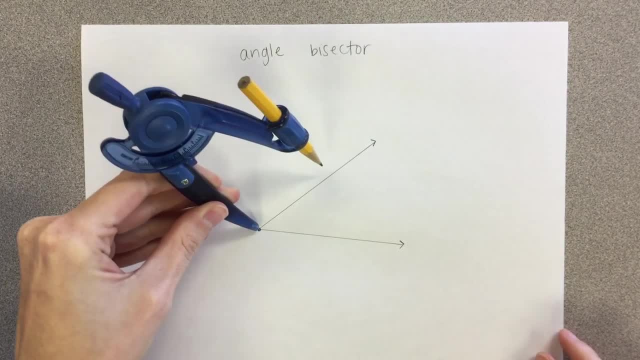 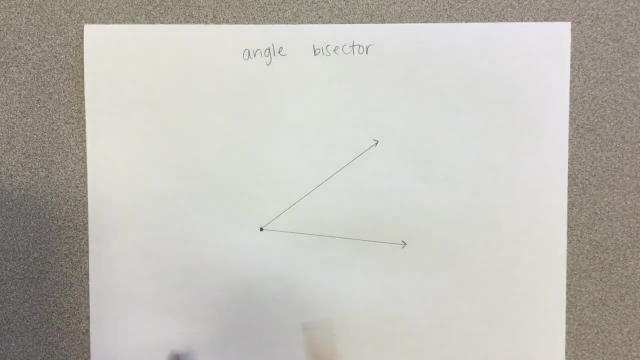 And it really doesn't matter how big I draw the circle. I'm going to choose to draw it about this big And I could draw the entire circle, or I really only need the points where it intersects with my angle. So I'm actually just going to draw part of the circle. 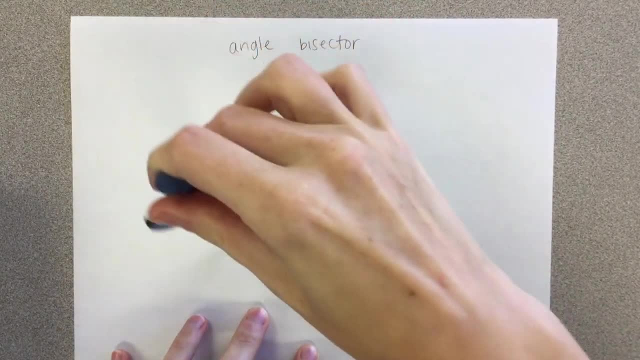 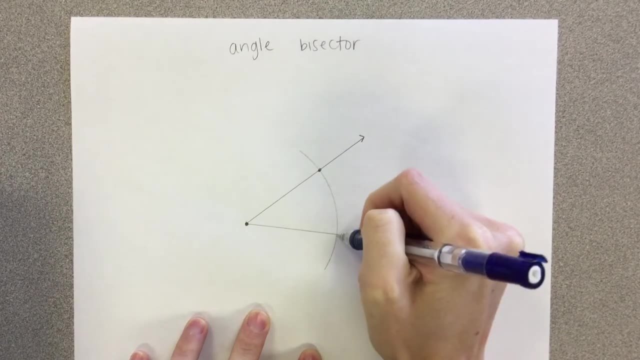 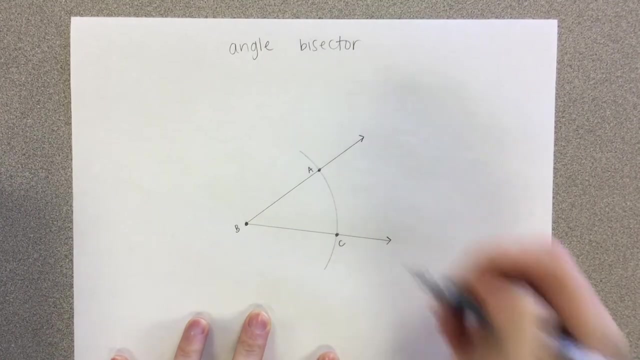 So again, I want to center this at the vertex And I'm just going to draw part of the circle And so it intersects the angle at these two points. I'm going to go ahead and label all these points, So I'll call this A, B and C. 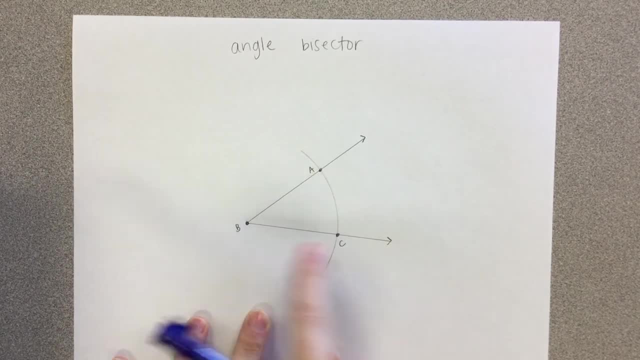 So this big angle that we're bisecting is angle ABC. What I'm going to do next is I'm going to draw a couple more circles using my compass, And so what I'm going to do is I'm going to draw a circle centered at A. 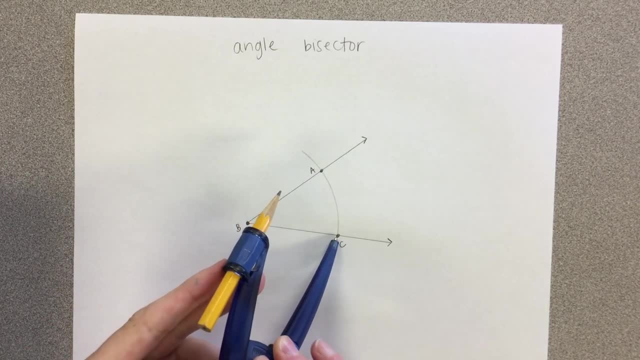 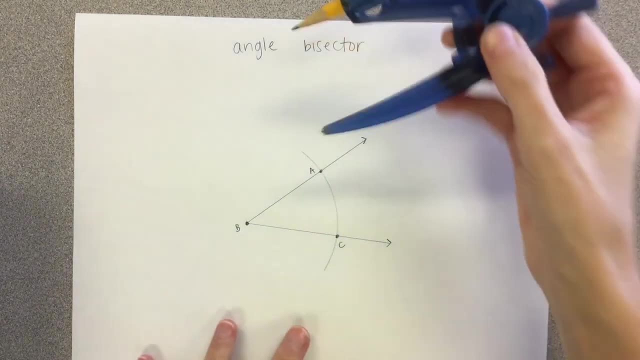 And then after that I'm going to draw another circle centered at C. I'm going to find where those circles intersect And that's going to help me find the angle bisector. So I'm going to start with my circle centered at A. 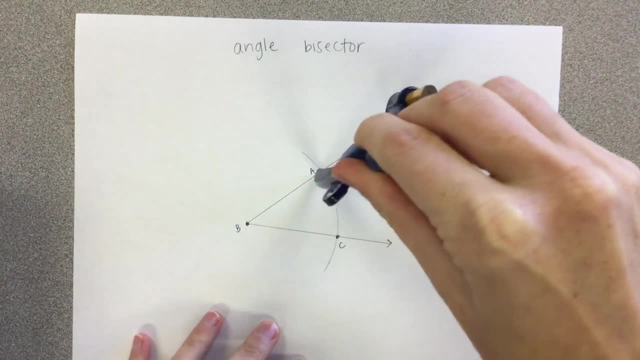 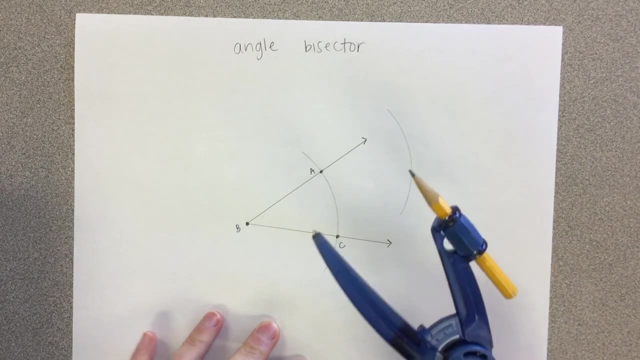 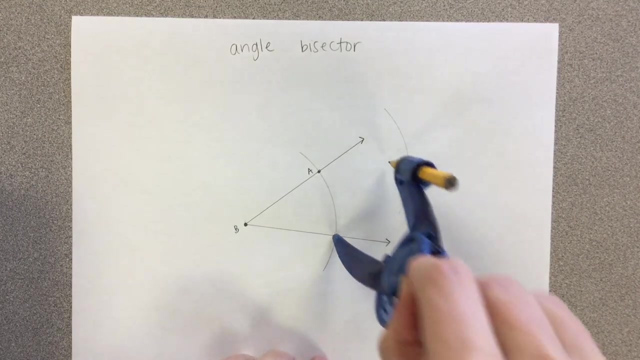 And again, I could draw the whole thing, or I know I really only need a little piece of the circle, So I'm just going to draw part of it. I'm going to keep my compass at the same radius here And I'm going to draw another circle centered at point C. 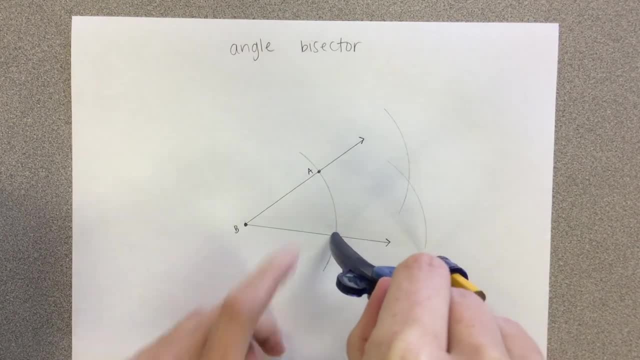 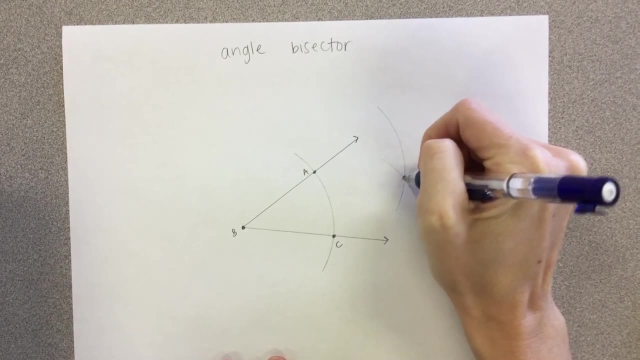 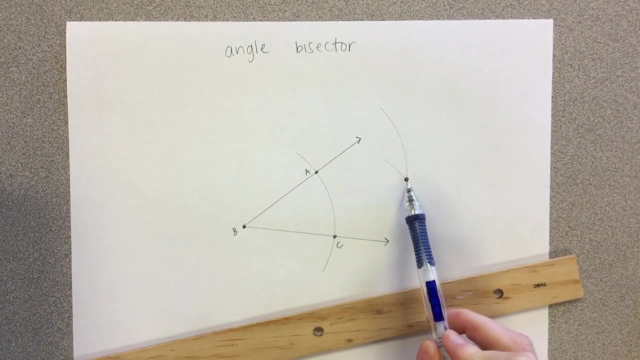 And I just really need this intersection point where these two circles cross. So again, I'm just going to draw part of those. So this point right here, If I take my straight edge and draw a line segment from B to this point over here. 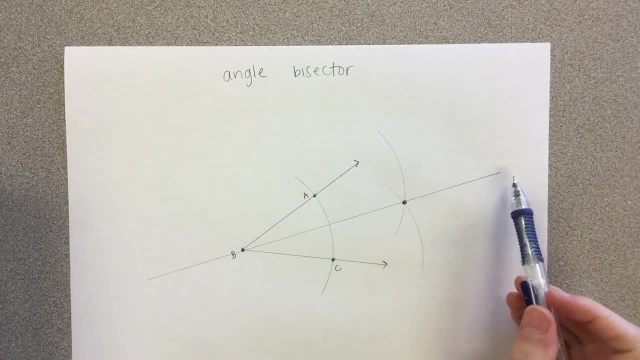 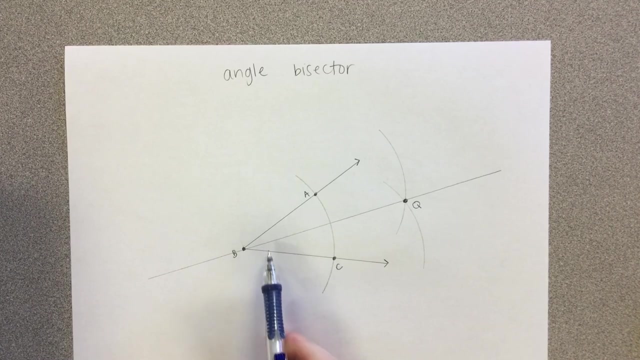 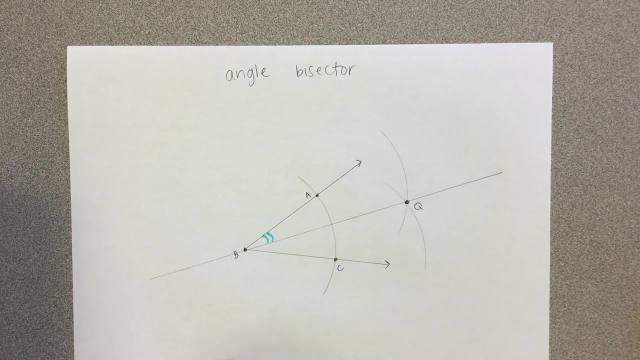 This line is an angle bisector. I'm going to label this. I'll pick letter Q for that. So this big angle, angle ABC, is now cut into two smaller angles that are the same size, That are congruent, And so I'm going to put little congruent markers in this angle. 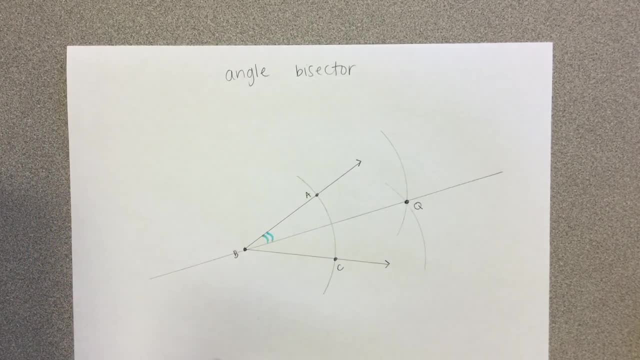 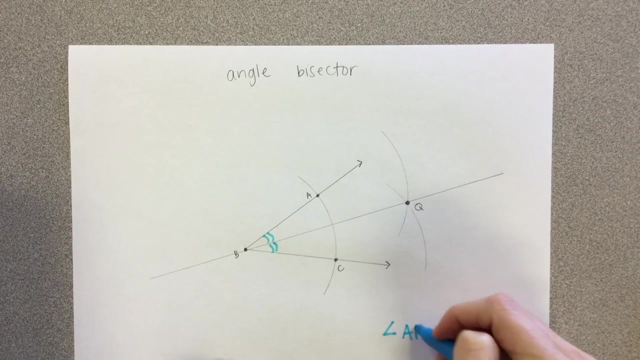 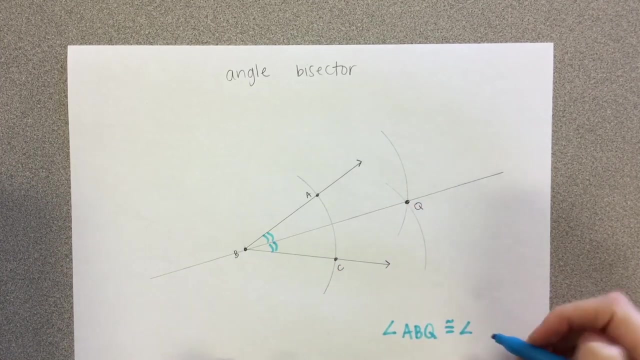 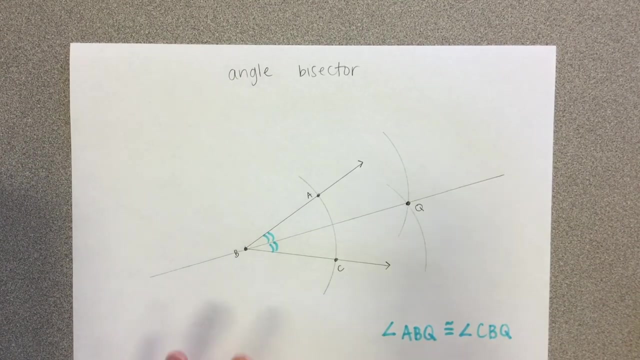 That could be called angle ABQ And it's congruent to this side over here, which could be called angle CBQ. So I could write a congruent statement to say that angle ABQ is congruent to angle CBQ And this is what is known again as an angle bisector. 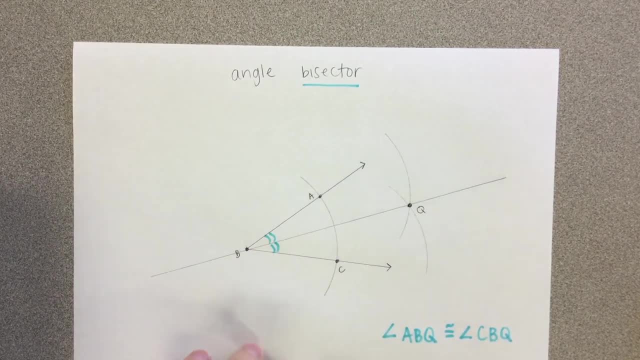 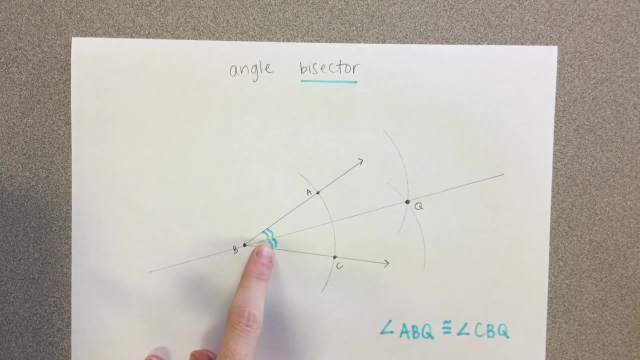 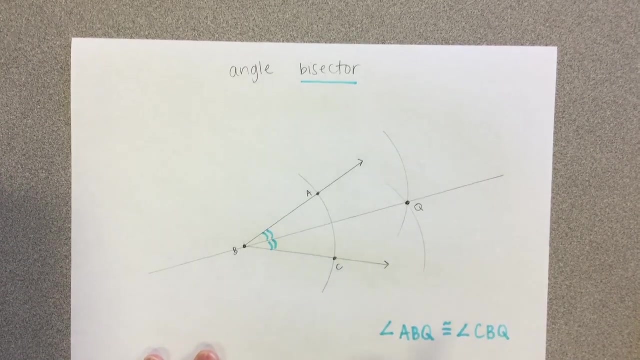 Cut this big angle into two smaller angles. So another thing that I could write is I could say that one of these smaller angles is half the size of the bigger angle. So I could say something like the measure of angle, and I'm going to do one of the smaller ones. 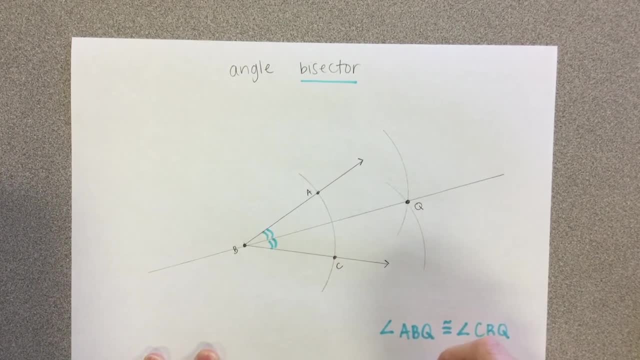 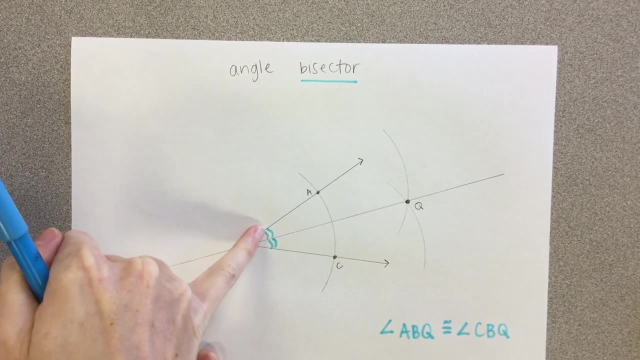 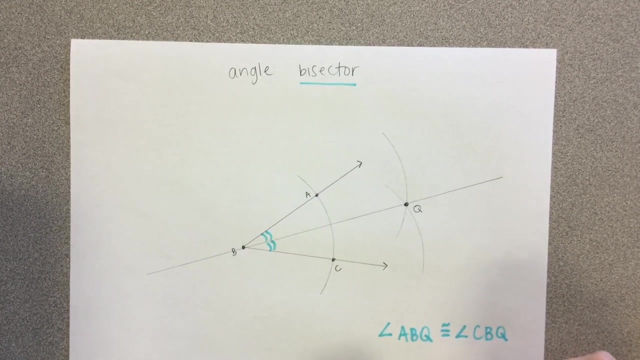 So angle ABQ, This angle angle ABQ. So this part up here, This part up here is half the size of the bigger angle ABC. So I could say that the measure of the smaller angle is equal to half the measure of the bigger angle ABC. 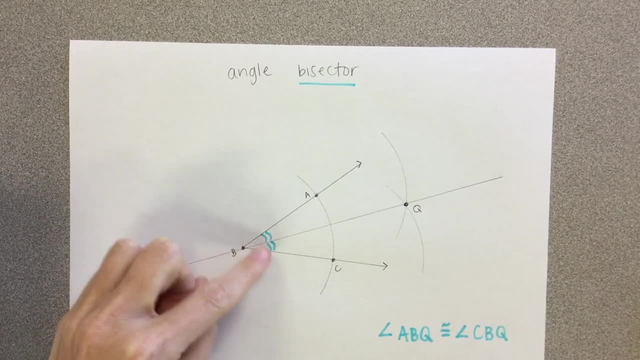 Now, one last thing I can do to check to see that these two angles really are congruent- And again, I'm not going to measure, so I'm not going to use a protractor. What I am going to use, though, is another little piece of paper. 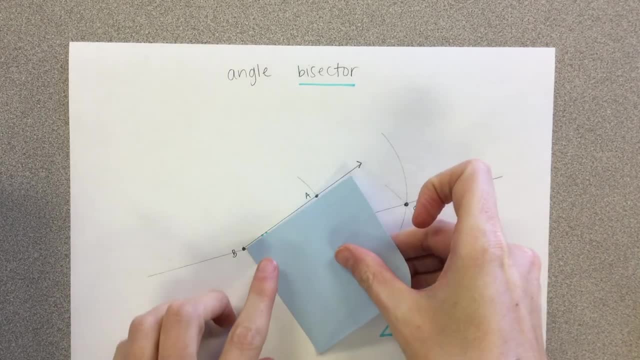 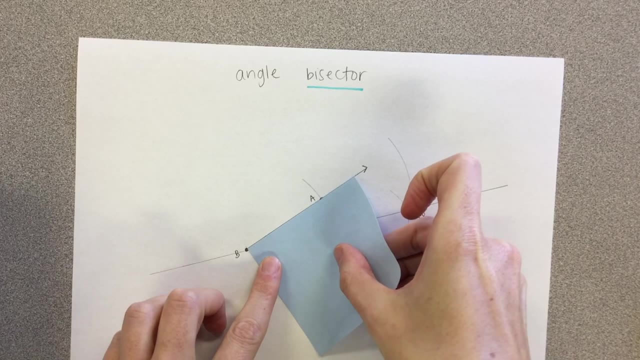 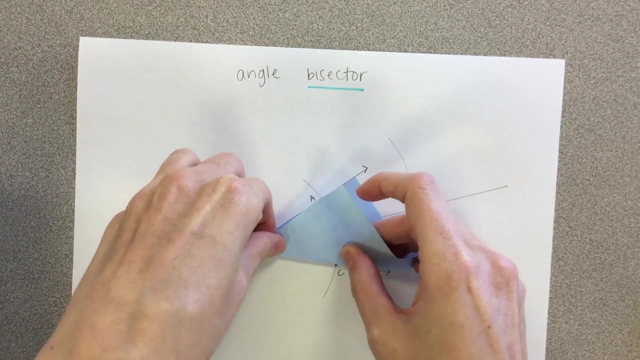 And I'm going to end up cutting this paper to the size of this big angle, angle ABC. And so, to help me do that, I'm going to line up a corner with the vertex and along one of these rays And I'm going to fold my paper along the other ray of this angle. 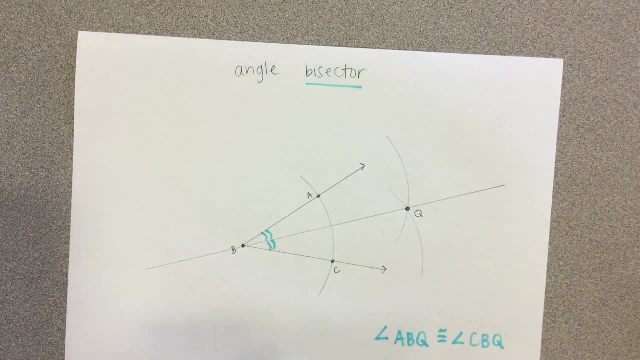 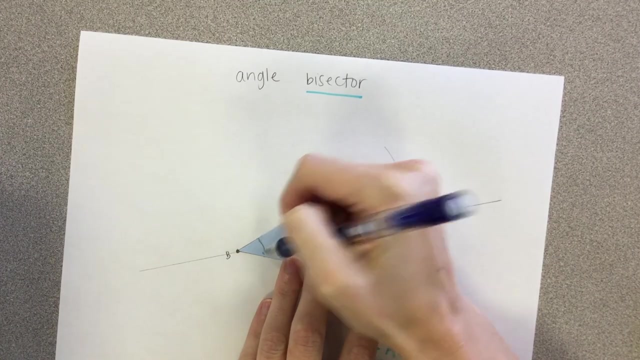 And then I'm going to cut along my fold And I'm going to try to cut as precisely as I can. Alright, So this corner, and I'll go ahead and mark it, This is the measure of our original angle. angle ABC. 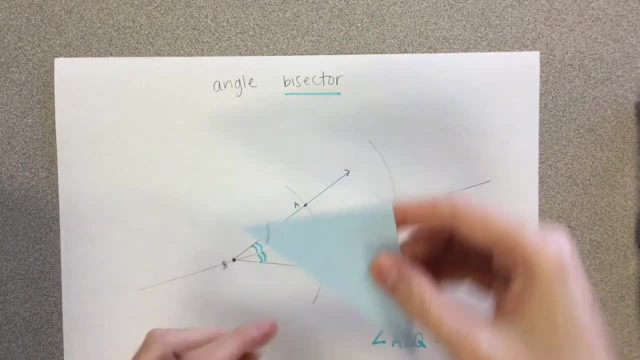 So if I fold this angle in half, So I'm going to take this piece of paper and fold it right down. So I'm going to fold this piece of paper and fold it right down. I'm going to fold this piece of paper and fold it right down. this vertex.